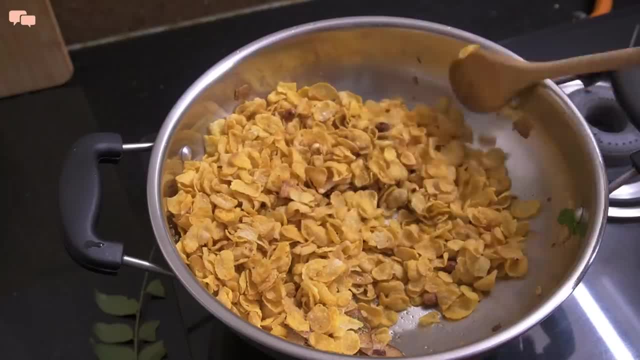 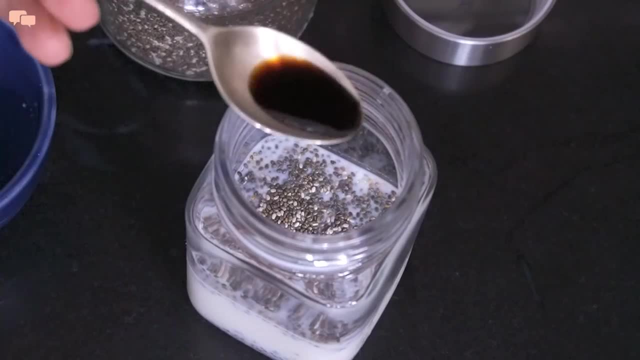 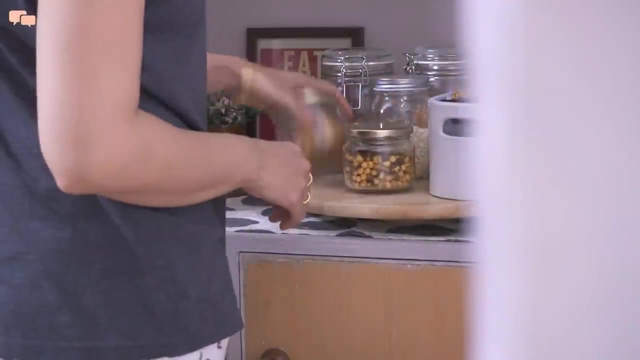 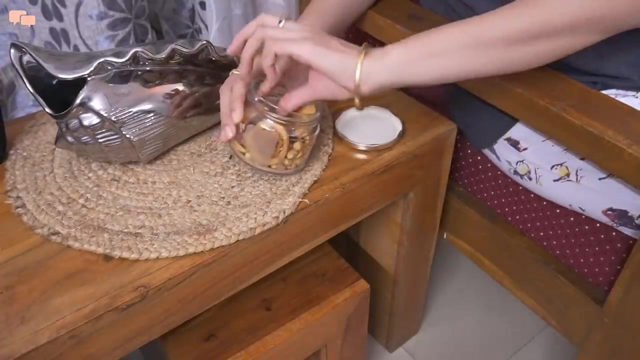 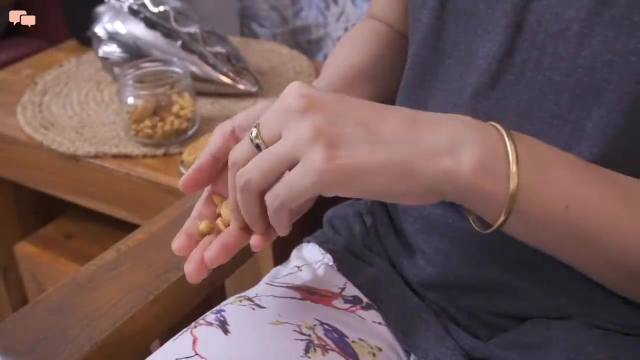 Hello everyone and welcome back. My snacking situation was not appetizing lately and since everyone in the house needs small eats every now and then, I decided to dedicate this weekend entirely in making easy, healthy and mouth-watering snacks that we as a family can enjoy. for the rest, 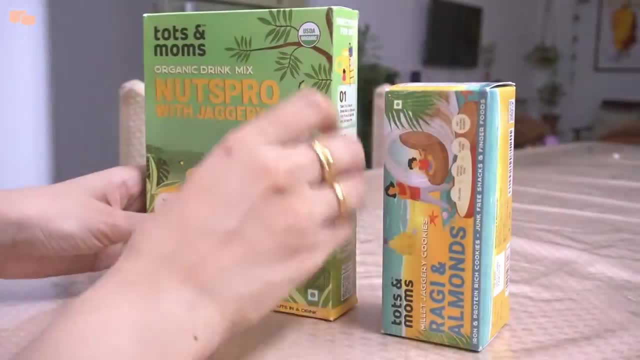 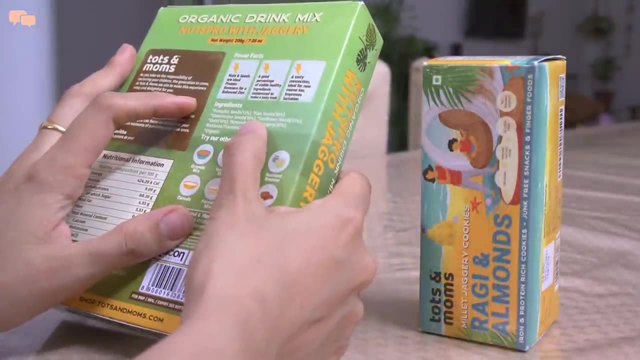 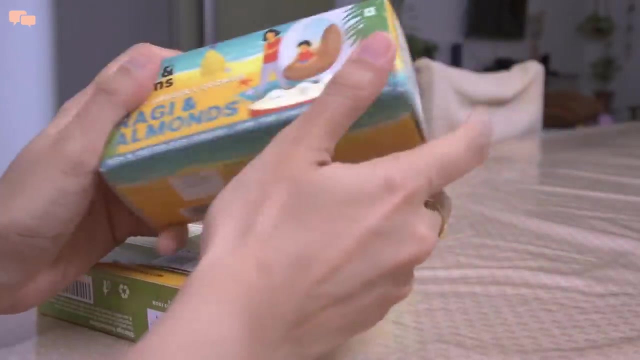 of the week For a variety of healthy snacking options. I was happy to collaborate with Tots and Moms Foods. In our household it is the most trusted organic food brand as they provide a wholesome snacking experience with the goodness of superfoods From millet to whole grains nuts. 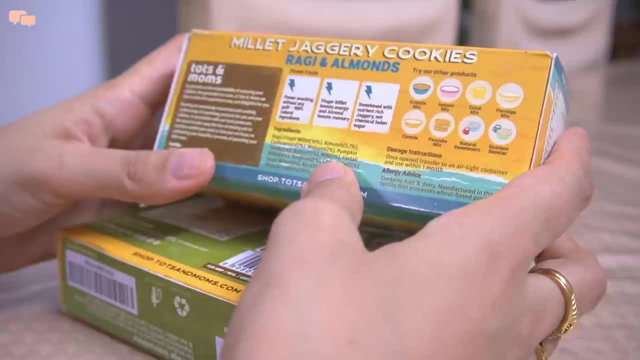 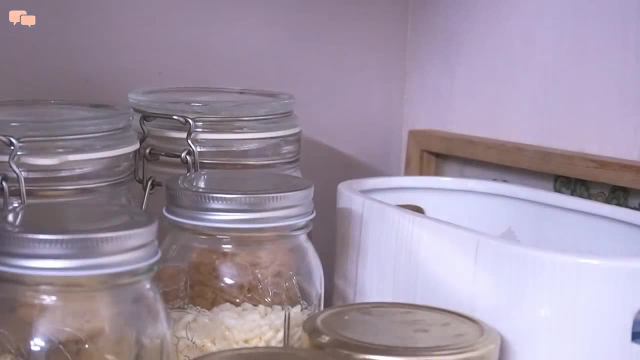 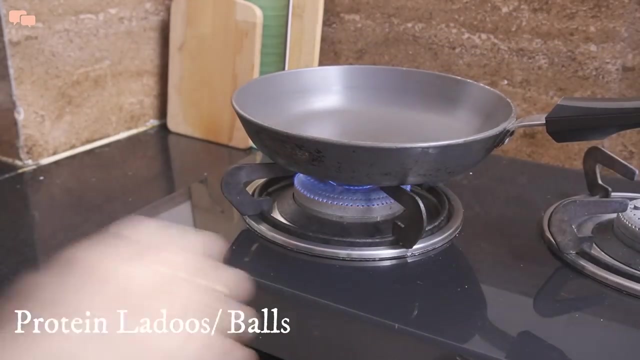 to seeds, to jaggery. their products are a complete health package. Their cookies and nuts pro health drink are a staple in our house, and while cookies will wait till tea time, I found a deliciously different way to use the health drink mix to make protein laddoos. Making laddoos always takes me. 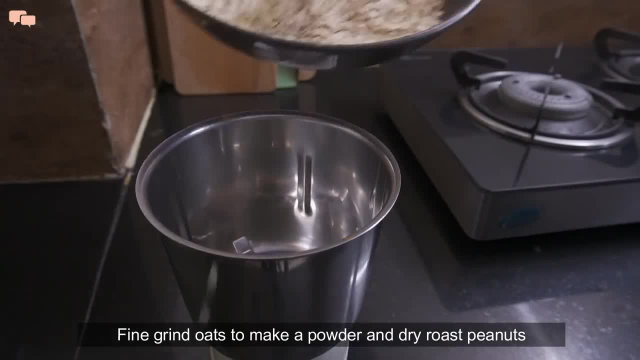 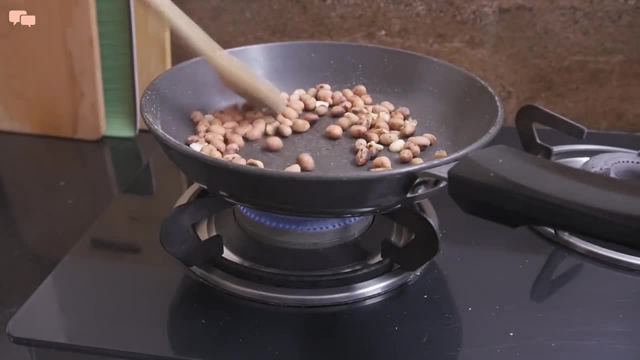 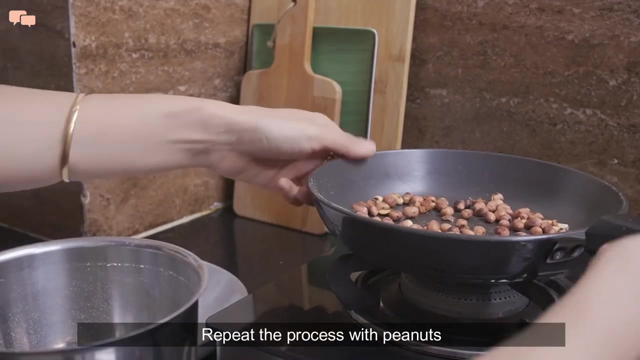 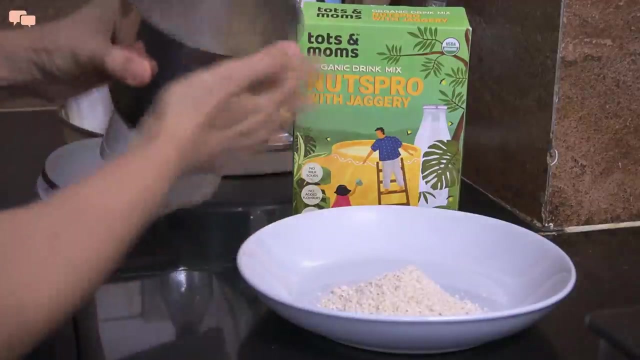 back to my childhood. Different laddoos in different seasons was a complete family affair. The habit continued well into adulthood, and now I know why They are not just super delicious but are visually appetizing as well. In making these protein laddoos, I kept the recipe very simple, Starting with oats to give them shape. 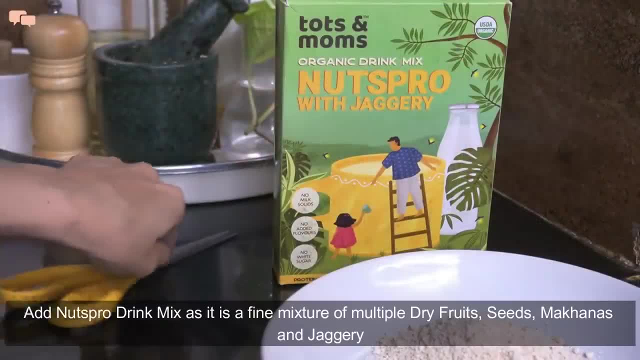 and then added peanuts for the goodness of proteins and also to bind them together. Then I added the star of the show, this nut and nut pro health mix. This nut and nut pro health mix is a great snacking snack for kids and adults. 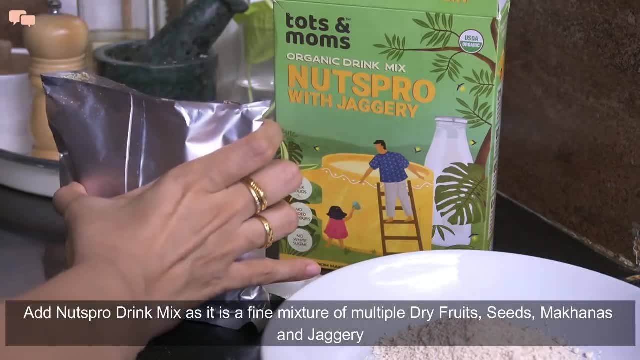 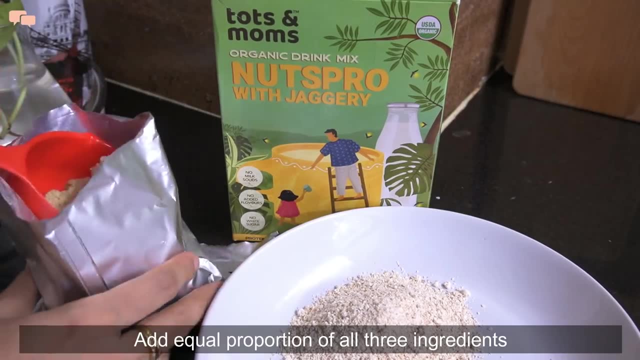 Then I added the star of the show. this nut and nut pro health mix is a great snacking snack for kids and adults. Let me give my opinion of the design part to you. I shared it in my next video and I'd like to see what you think about this in the comment section below. 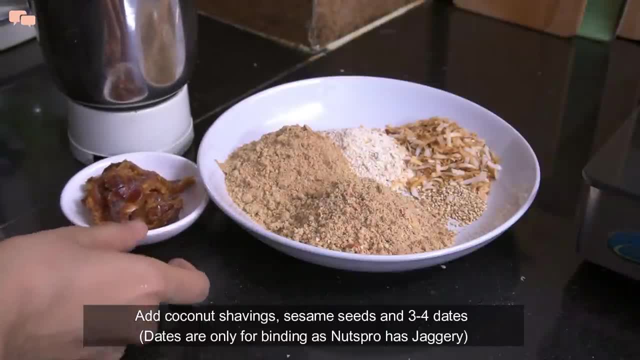 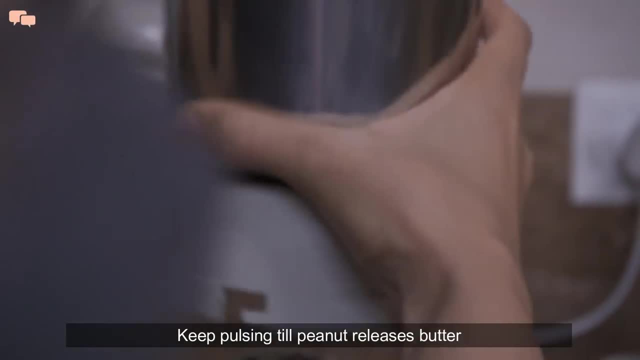 And now that I am very satisfied here, let me share a complete recipe of beans and nuts. pro Health drink. strawberry flavourную nation was made with good quality Pennsylvanian dates. It saved me all the time and effort in making a fine mix of multiple nuts and seeds. 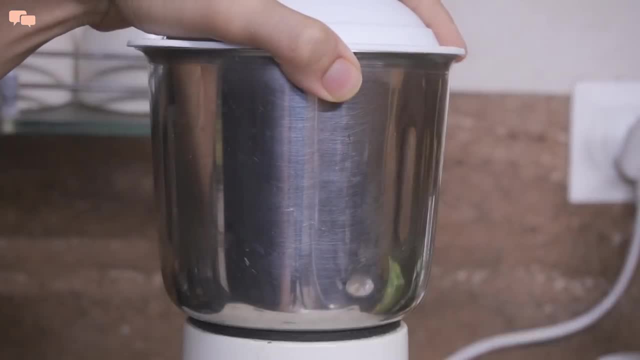 At the end I'll add coconut and few sesame seeds for great taste, followed by dates, which again will bind the whole mixture together. I'll put everything in a mixing jar and pulse the mixer till everything starts coming together. Wasn't it a great health drink. 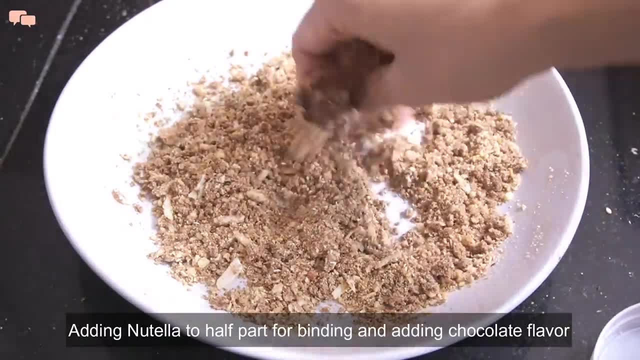 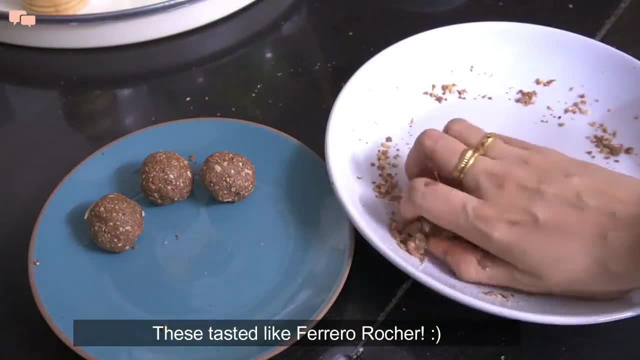 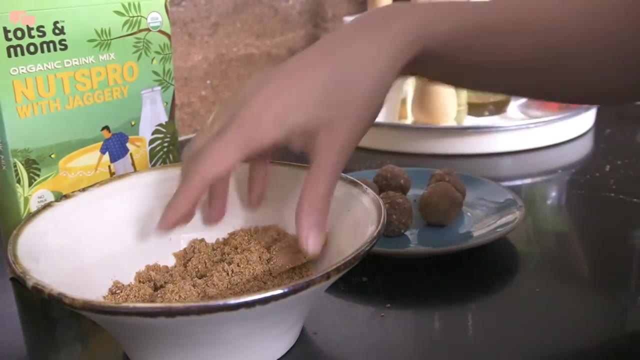 Bea politicians, promiseals are mentioned. great health combo. I also made a Nutella variant, which was super yum as well, and this one was specifically for Ruthvi. Multiple dry fruits, seeds and makhanas from the Nuts Pro Health Mix: make these laddoos. 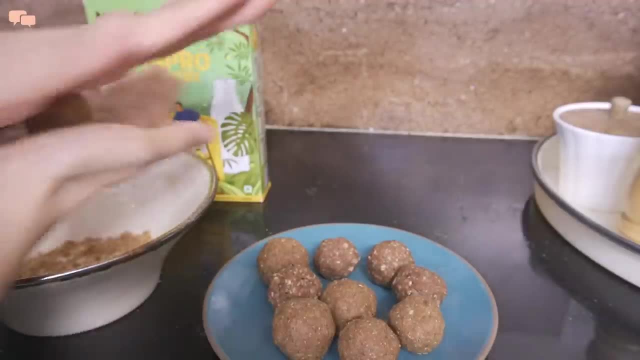 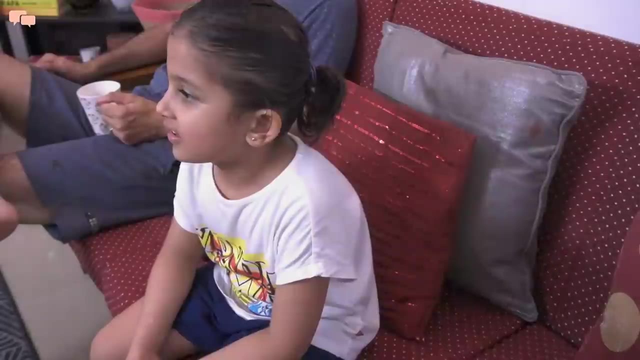 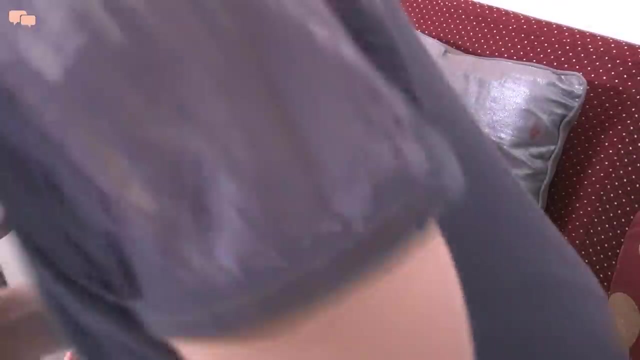 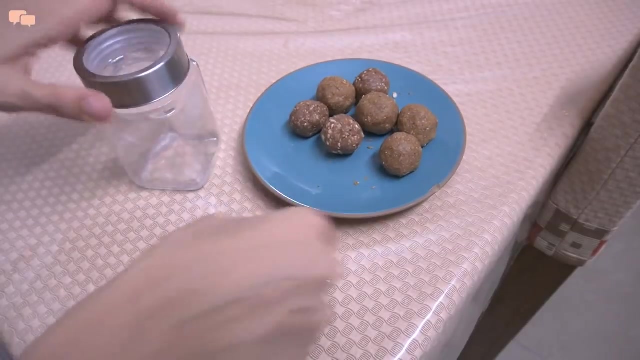 high in protein and rich in calcium and minerals. This surely helps in improving the immunity and the overall brain development. So here it is, a guilt free, absolutely healthy and easy to make snack option which is ready in a jiffy. It was the testing time and we all pounced on them. and just as I thought, 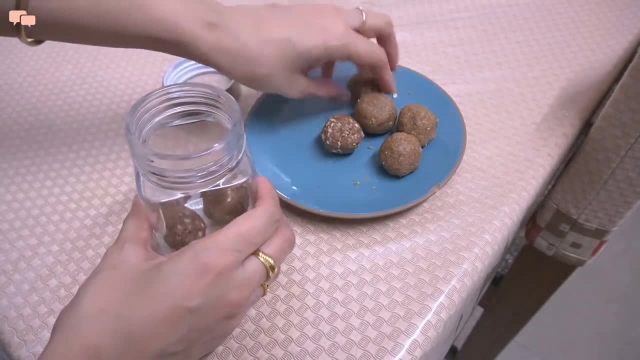 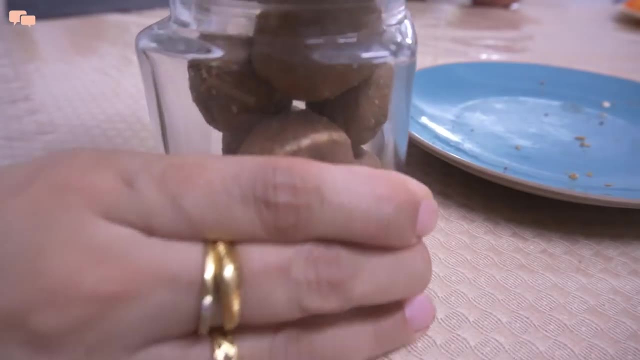 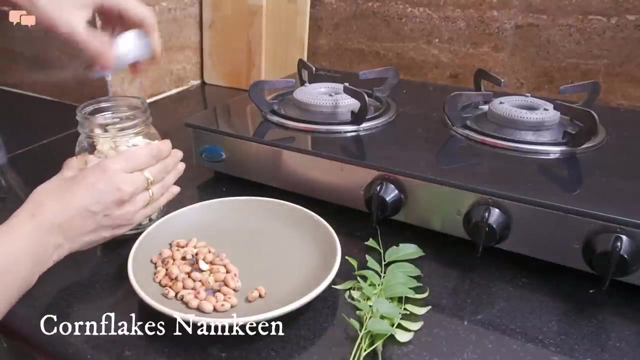 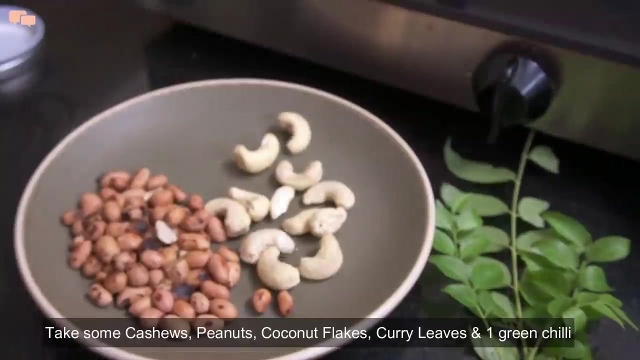 Ruthvi kept asking for more. All I regret that I made them in such a small batch, So lesson learned for the next time. Namkeen is another quintessential snack in the house. We at times even enjoy a handful along with meal as a condiment. But snacking on those store bought namkeen was filled with. 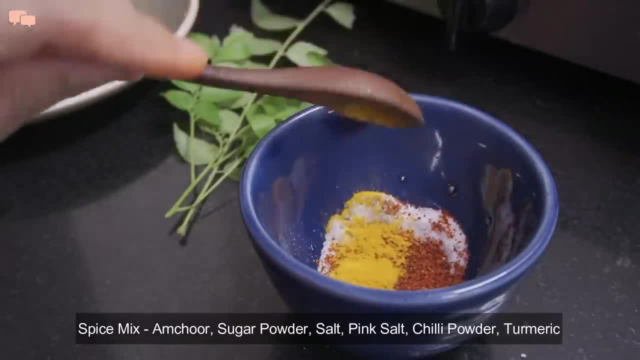 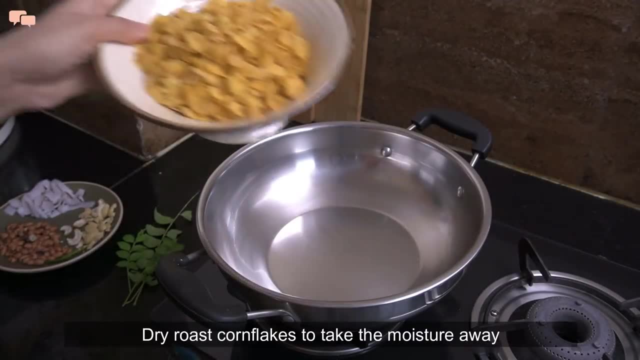 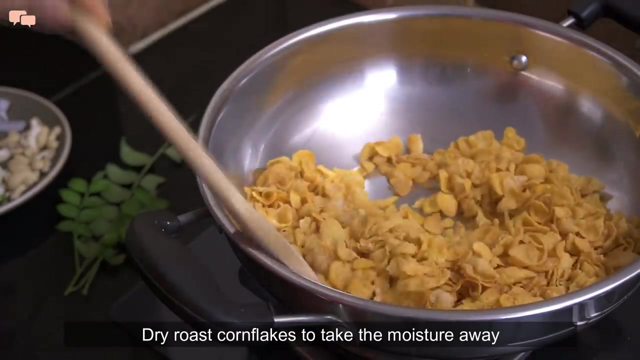 a lot of guilt. So I made some namkeen on my own, and cornflakes just came handy. I collected all sorts of fillings. It took me 10 minutes to prepare this easy and quick snack. Making homemade namkeen got me thinking that preparing food at home gives so much freedom. 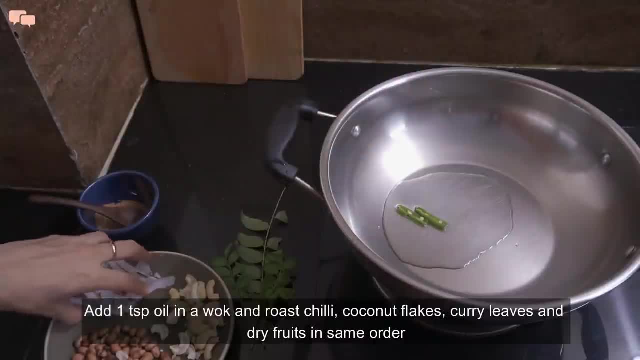 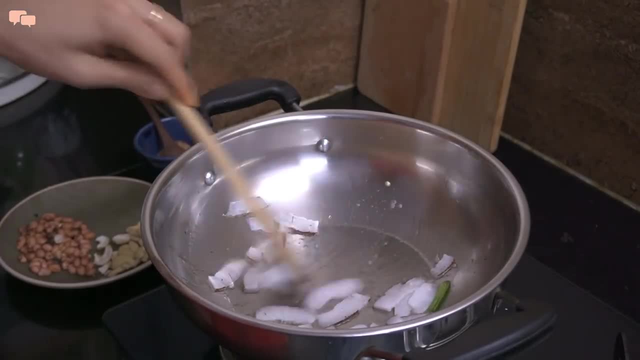 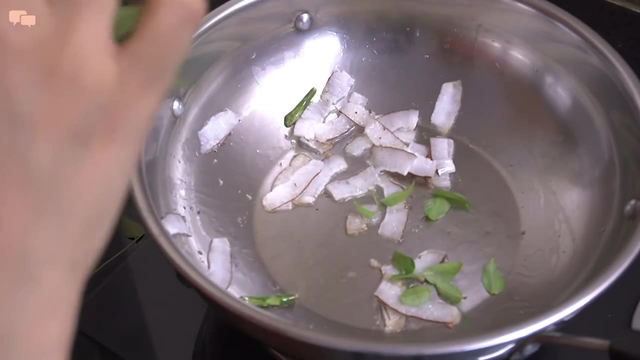 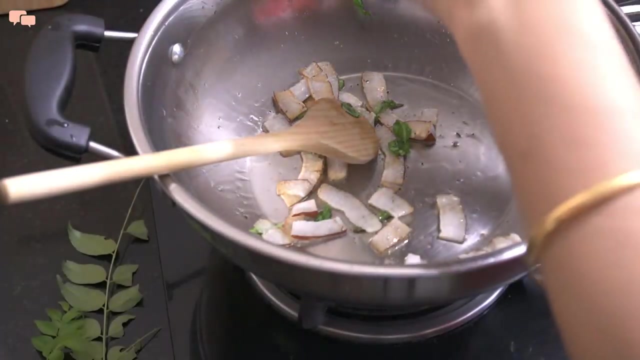 of customization and sense of relief that whatever you are eating is safe, nutritious and delicious at the same time. I slow roasted every item one by one to take the maximum moisture out so that the namkeen can last longer. I was super happy with the fact that by making snack at home, also made me utilize the existing 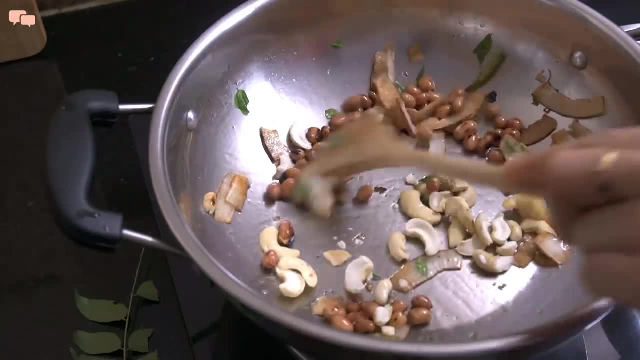 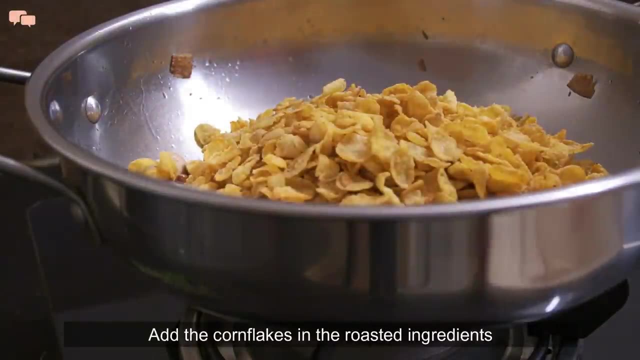 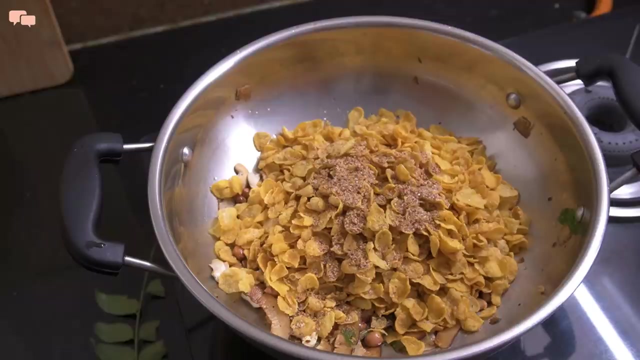 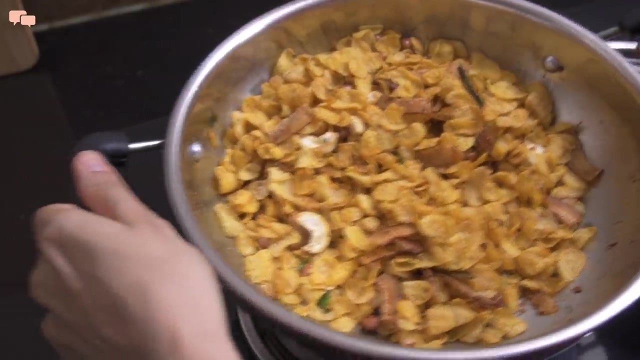 grocery items which was otherwise just lying and getting wasted. So overall, I got a nice kick to find more such creative and healthy way of consuming such items. The sound of these cornflakes namkeen was appetizing in itself, And once everything is well combined, don't forget to give it a taste and adjust the spices. 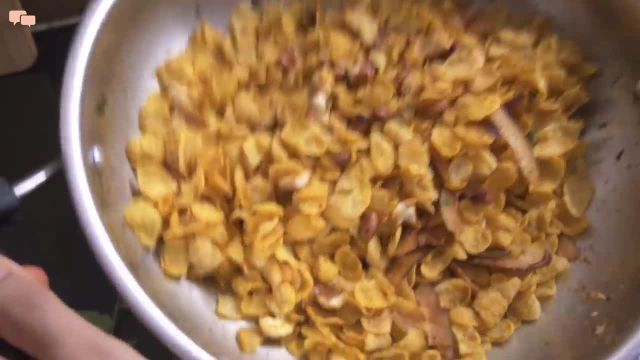 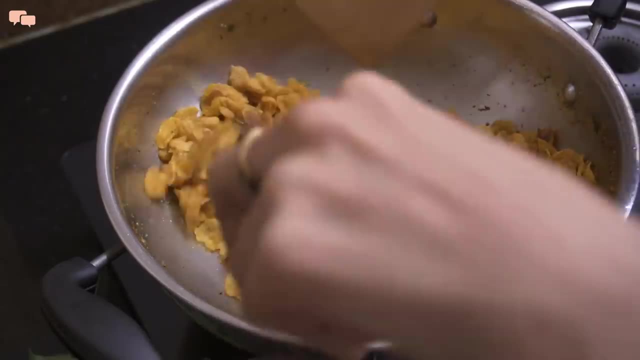 as per your liking. Have you guys also made cornflakes namkeen before? Let me know how else can I take it a notch higher? Or any other snack that is healthy and mouthwatering at the same time? Your suggestions always help in improving this experience. 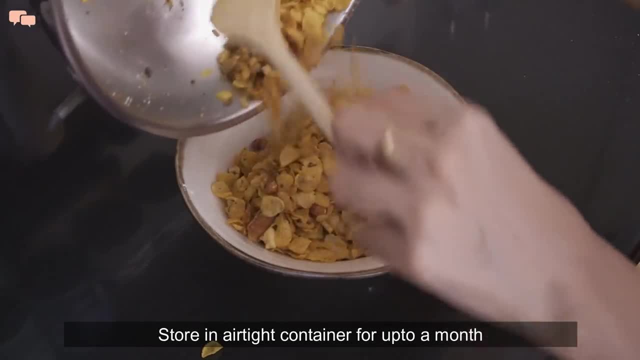 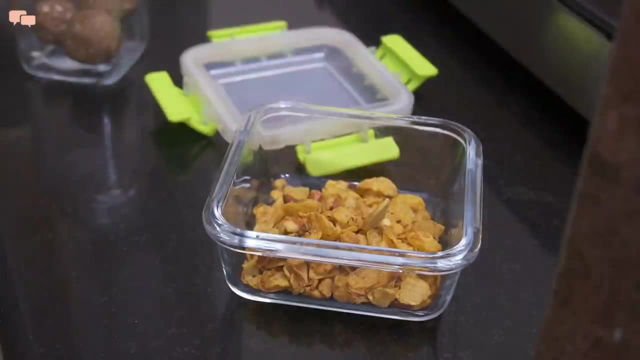 I hope you enjoyed this video. If you did, please share it with your friends and family. I will see you in the next one. Bye. A perfect snack for tea time, office lunchbox or time when you just want to indulge in some. 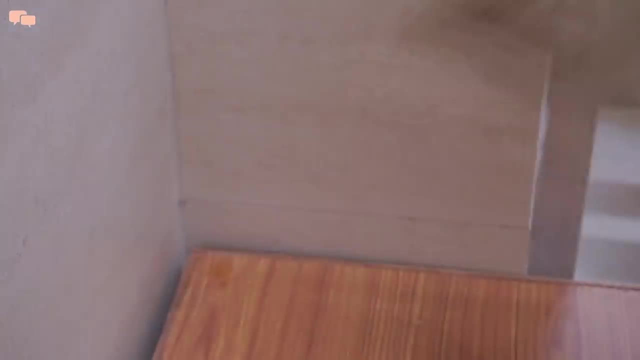 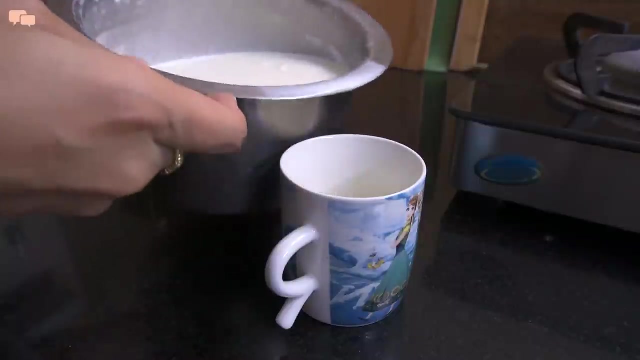 crunchy, spicy snacking. Evening tea time is also Ruthvi's milk time And, as I try to find ways to add more nutrition in her diet, instead of giving her plain milk I prefer adding the Nutspro health mix. I hope you enjoyed this video. If you did, please share it with your friends and family. 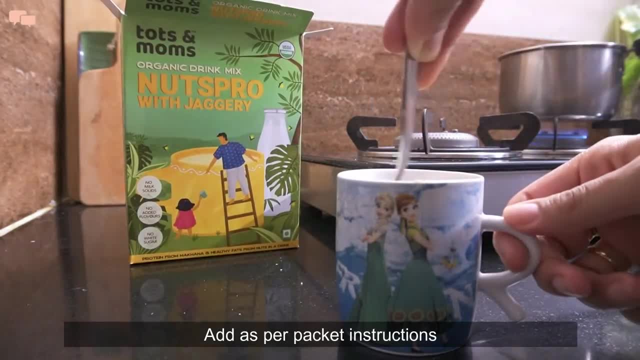 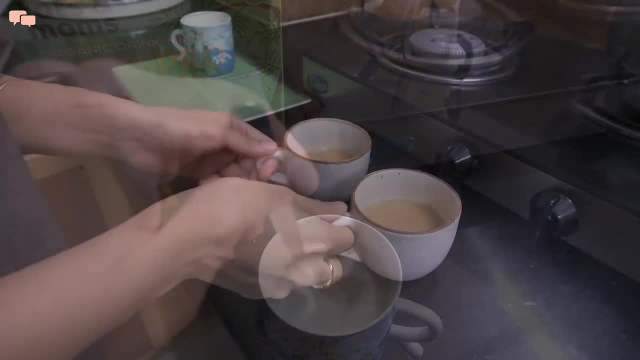 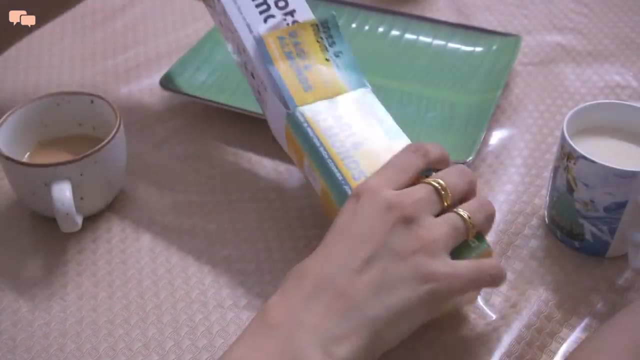 As a growing kid, she needs more calcium and improved immunity. It also gives me a lot of satisfaction that she is getting more nutrition without any out-of-the-book effort. And talking of reducing the effort, these Millet and Jaggery cookies from the Tots and 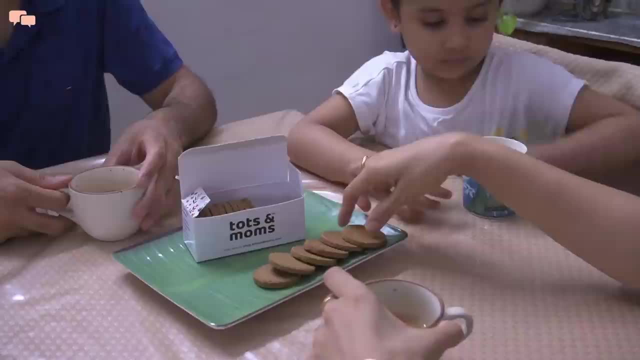 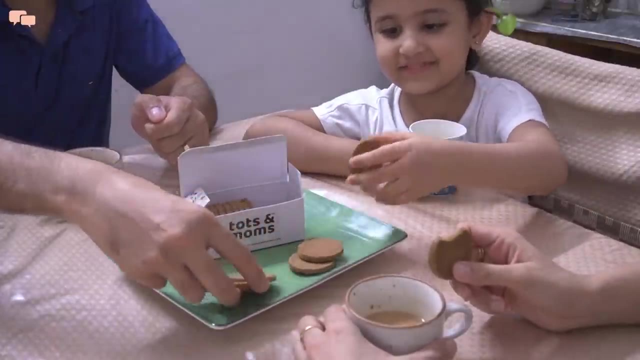 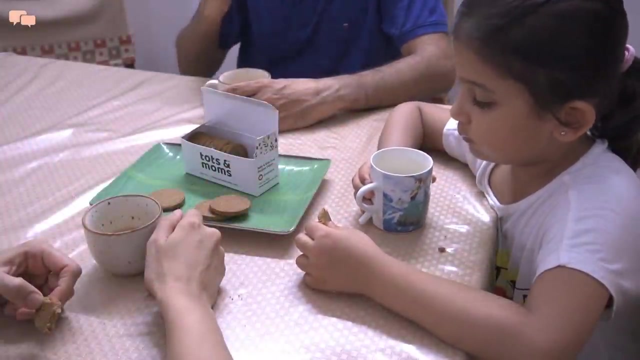 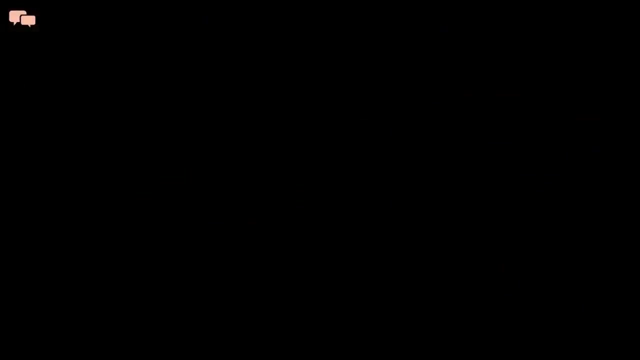 Moms are just the right snacking option at our tea time. Rich in iron and protein, these junk-free snacks are awesome And they are always welcoming. Above everything, it is fully organic and preservative-free. Easy to grab, organic, yet tasty treat, Isn't it amazing? 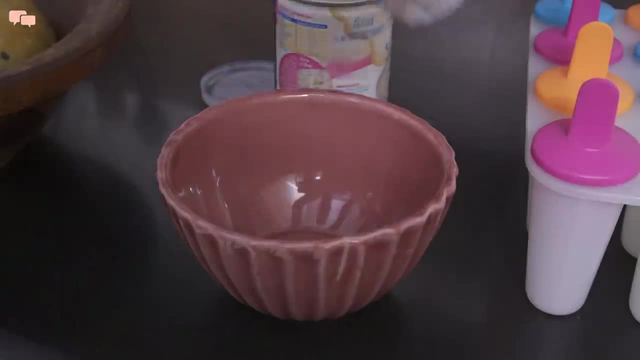 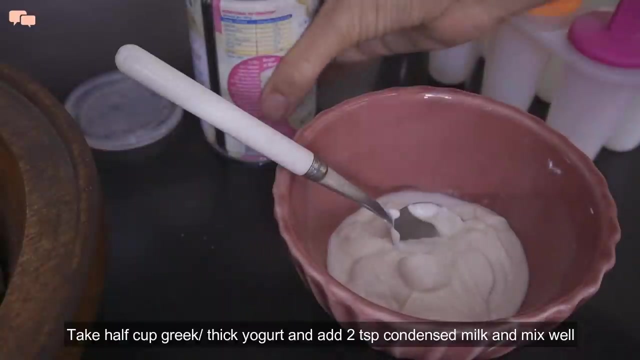 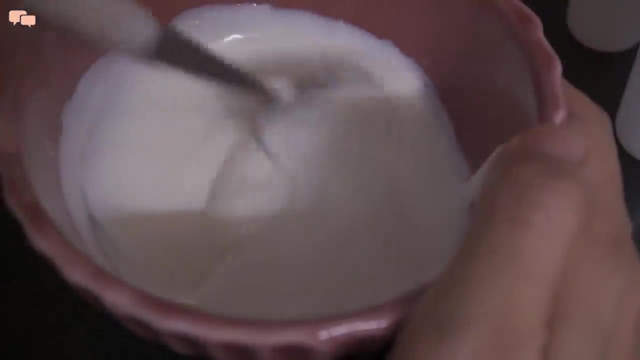 Next is everybody's all-time summer favorite Popsicle. I usually crave for sweets after dinner and lunches, so I thought, instead of ending up eating some unwanted sugary treat, Let's make some healthier snack which can help me curb my sweet cravings along with. 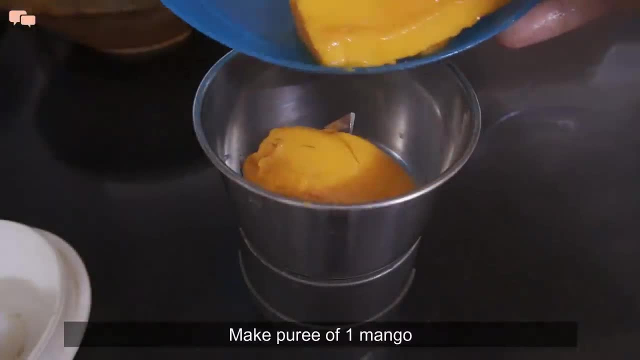 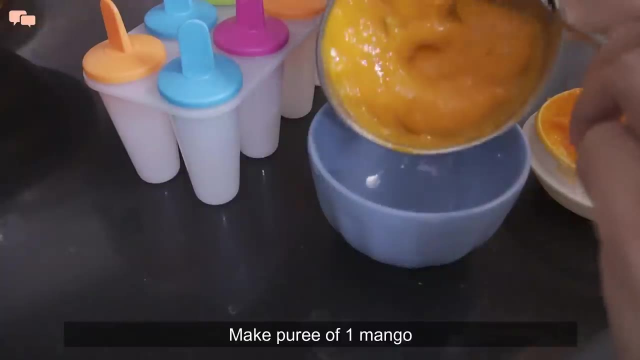 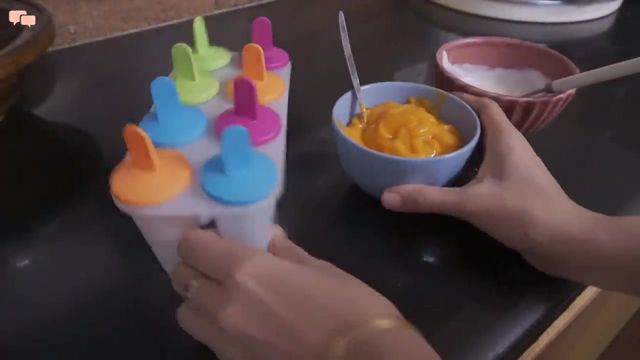 giving me nutrition. As I mentioned in my previous video, I am making the most of mangoes till the season lasts, So there were no second thoughts for Mango Popsicle. I chose the brightest mango of all. However, this quick snack does not need an extra effort. 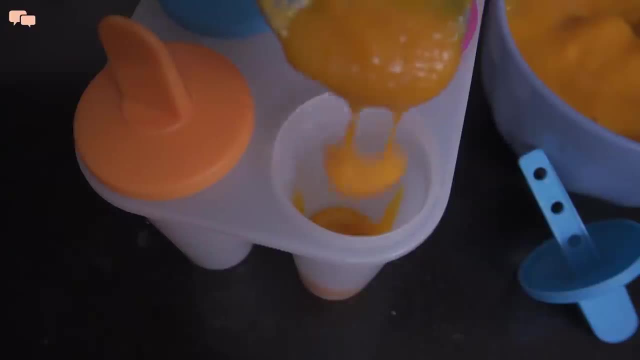 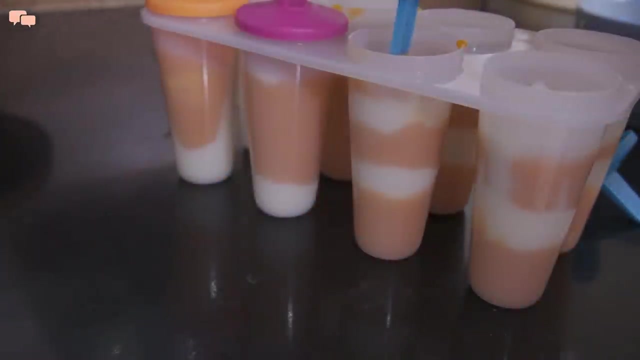 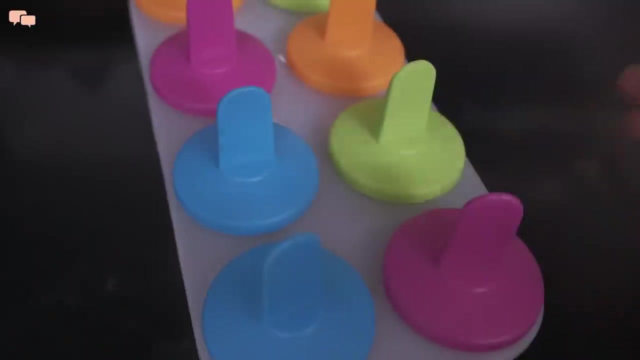 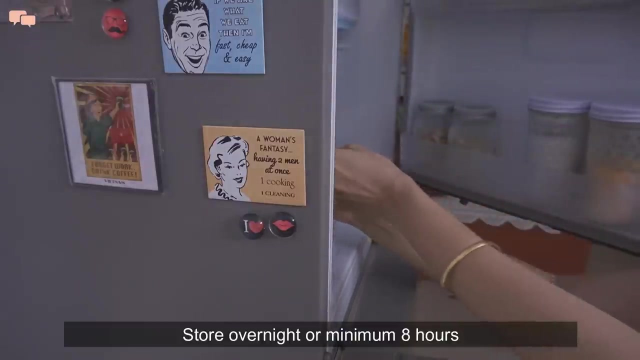 to catch the eye. It took just 5 minutes to do the preparation and assembling. it was great fun. Layer them as per your choice. This homemade yogurt popsicle without preservative will surely make the full house happy. As easy as this popsicle was to make, harder it was to wait for, but was indeed worth a. 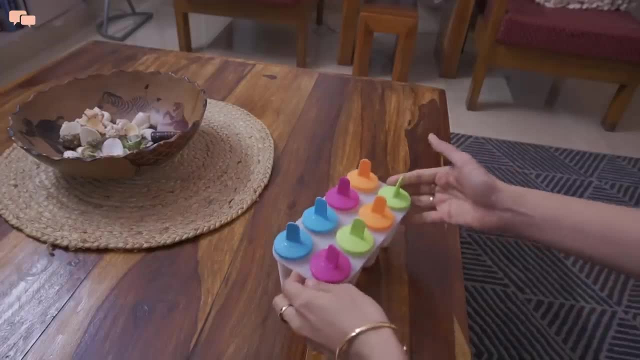 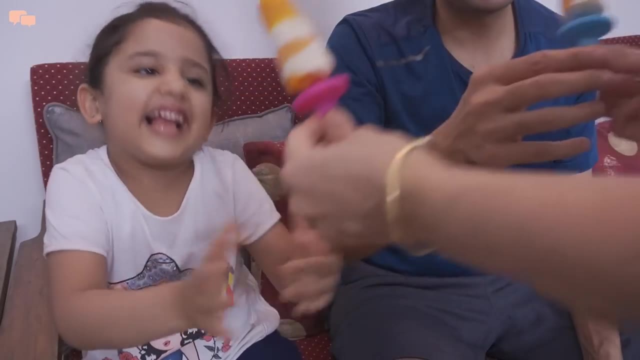 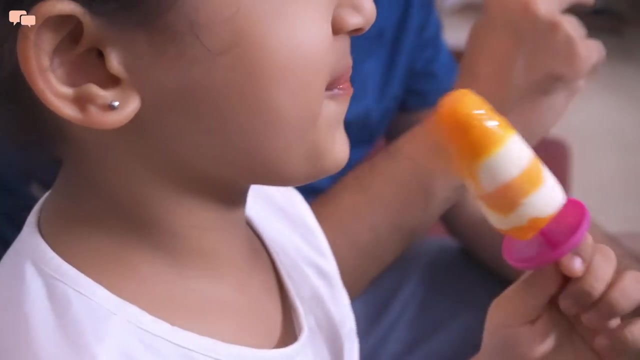 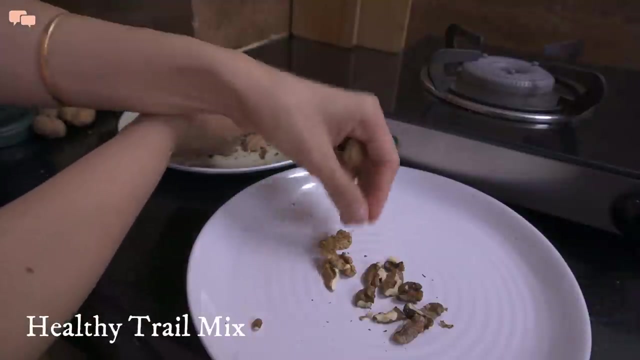 wait. Ruthvi's happiness after seeing the popsicles explained it all, So I decided that whenever she will have her friend's party, this fruity pulpy popsicle will surely be there in the menu. If you follow me on Instagram, you will know that last week my dad came visiting and he 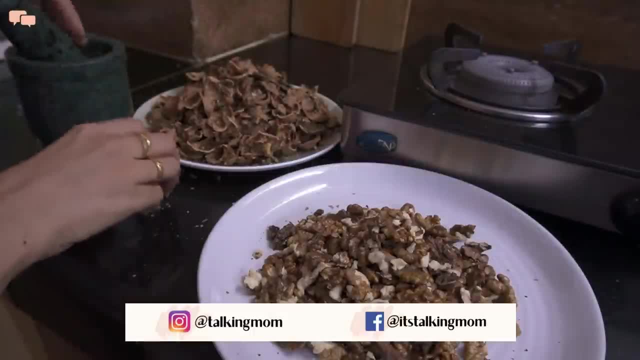 bought me a bag full of walnuts. That triggered me in making a trail mix of walnuts. This is the first time I am making a trail mix of walnuts. This is the first time I am making a trail mix of walnuts. This is the first time I am. 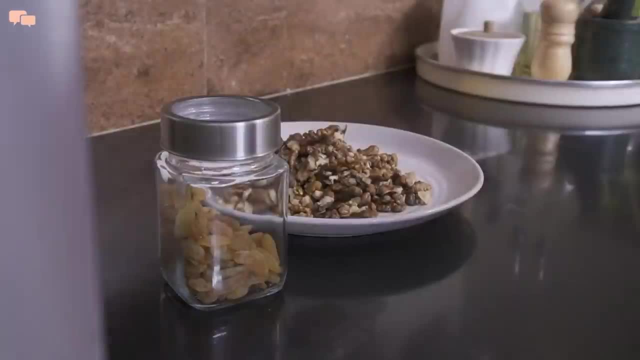 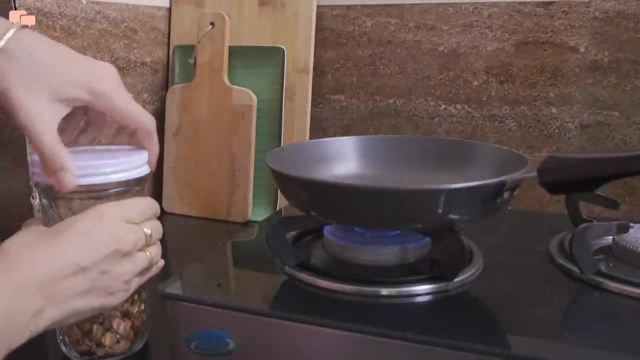 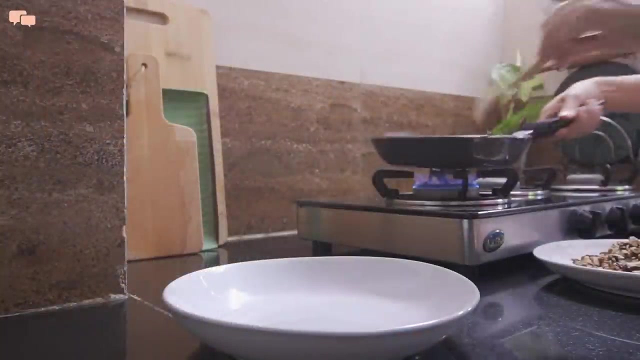 making a trail mix of walnuts, And this snack was specially for myself and Kartik's office. This one surely took a bit of an effort, but it was absolutely worth it. Nuts and seeds are an instant energy source and, when consumed in moderation, provides 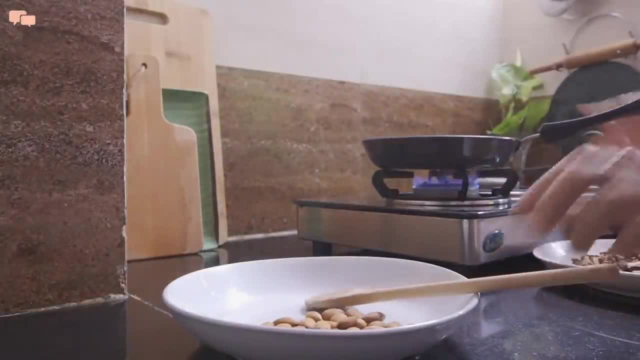 just the right amount of nutrition you look for every day. Picking nuts and seeds from their individual jars and eating them was quite a process. I had to be careful not to eat them, as they are very sour and they are very sweet. I had to be careful not to eat them, as they are very sour and they are very sweet. 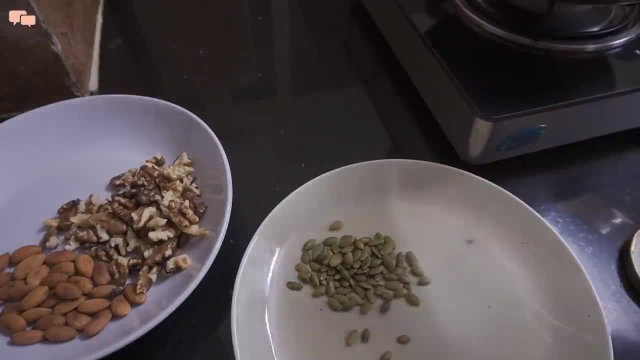 So I had to be careful not to eat them, as they are very sweet. So I had to be careful not to eat them, as they are very sweet. So I had to be careful not to eat them as they are very sweet. So the idea was fairly simple: to combine everything together in one jar by also making 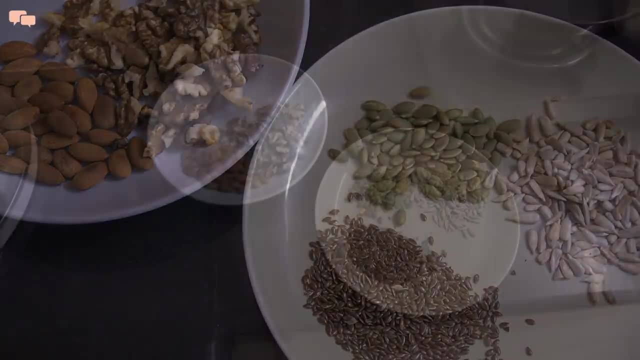 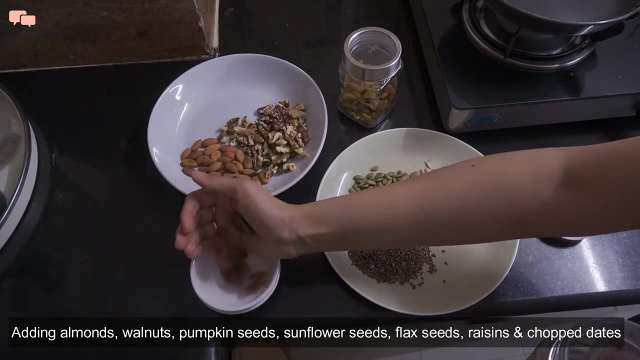 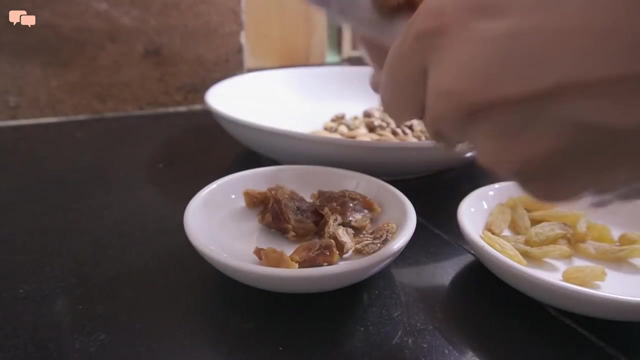 it appetizing because when things are prepared it's easier to consume. I dry roasted available nuts and seeds very slightly just to enhance the flavor and bring some aroma to it. But you may also choose to simply mix everything together and keep in an airtight jar. 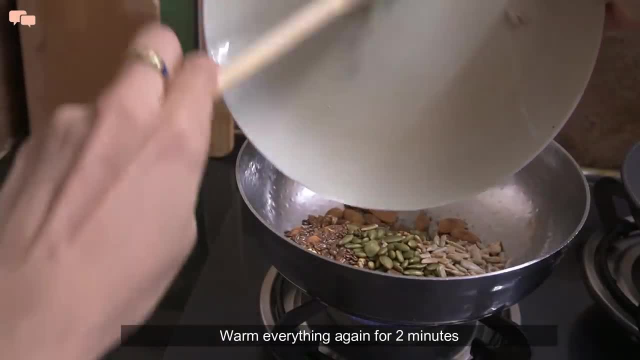 But you may also choose to simply mix everything together and keep in an airtight jar. But you may also choose to simply mix everything together and keep in an airtight jar. Healthy trail mix is basically a combination of some nuts, seeds, dry fruits or even fun. 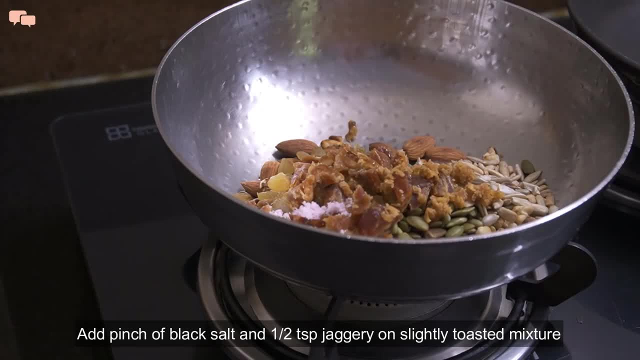 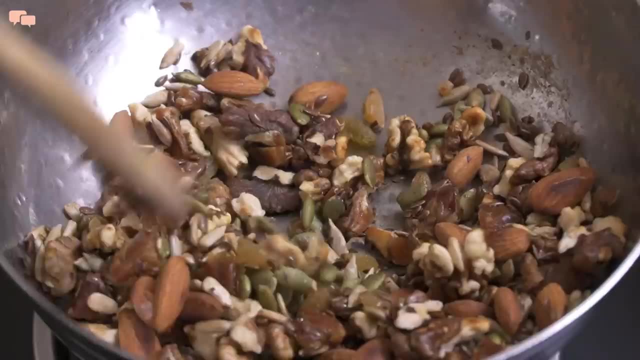 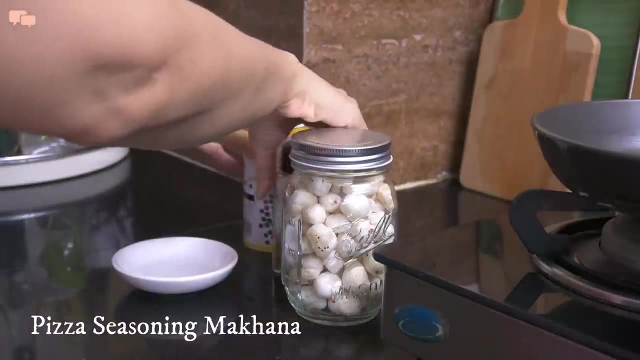 mixes like popcorn, choco chips, corn flakes, etc. Food choices differ in every household, so choose what suits your palate most. Talking about snacks and not talking about makhana is gross injustice. Healthy trail mix is basically a combination of some nuts, seeds, dry fruits or even fun. 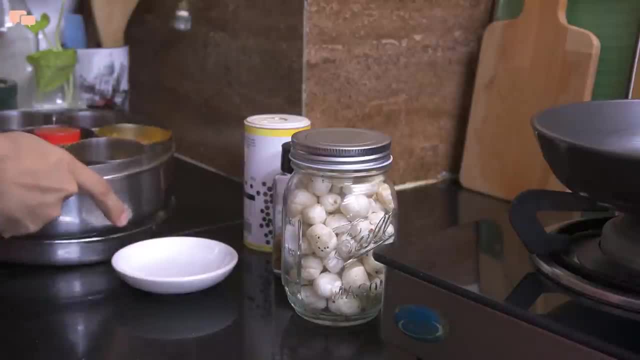 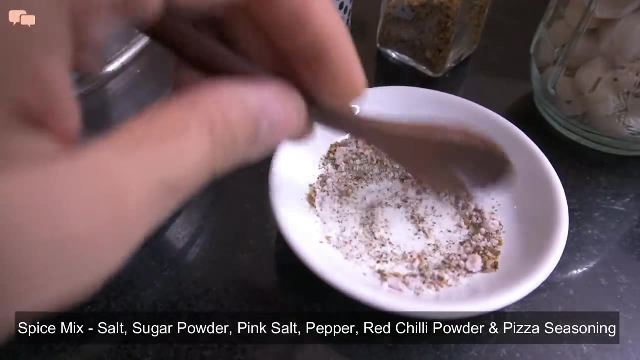 mixes like popcorn, choco chips, corn flakes, etc. and fibre-rich food makes the perfect snack, as it keeps us full till we reach the next meal. Since the original taste is so subtle, makhanas give enough ground to add as many flavours as you. 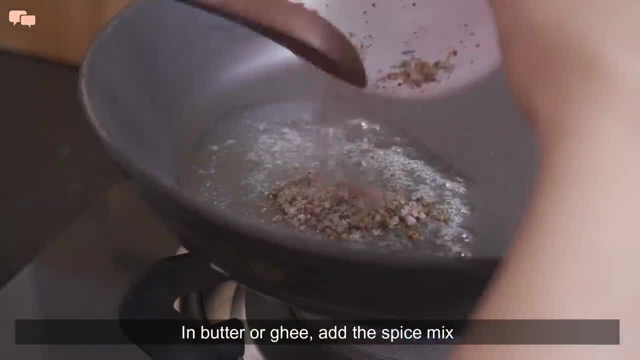 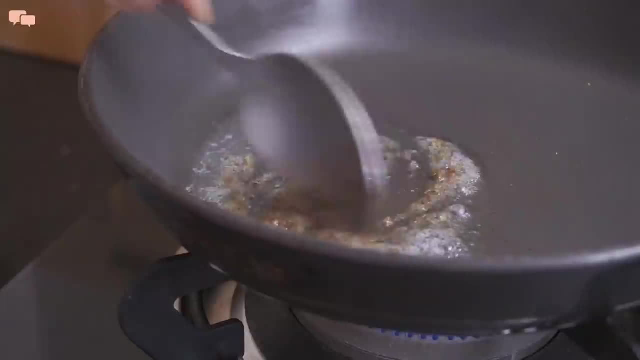 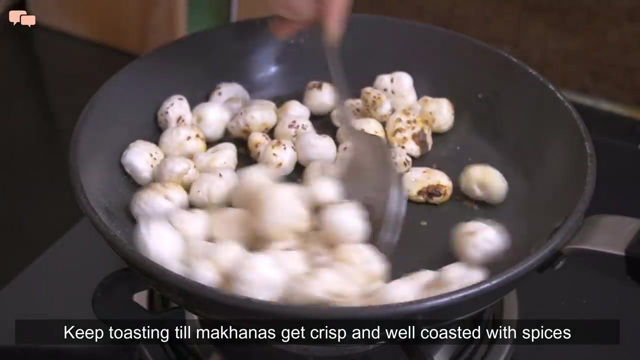 like Sweet, salty or spicy. the choices are fairly unlimited. Rather, if you have a tried and tested spice mix for makhanas, do share with me, because I love experimenting with different flavours, so that we never get bored of this quick to make and healthy snack. I usually make it in. 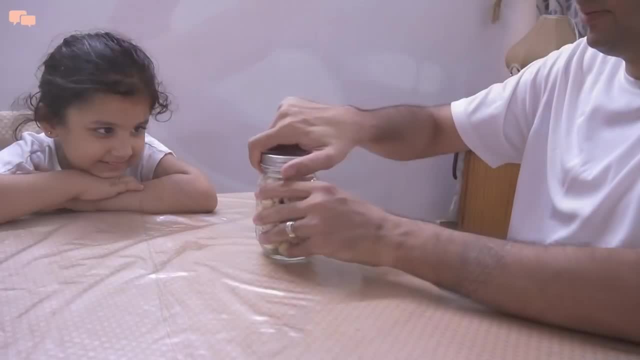 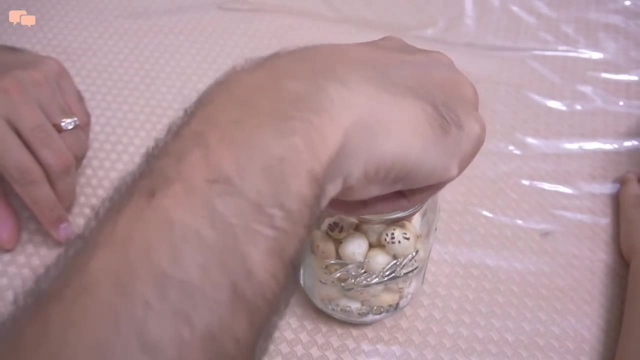 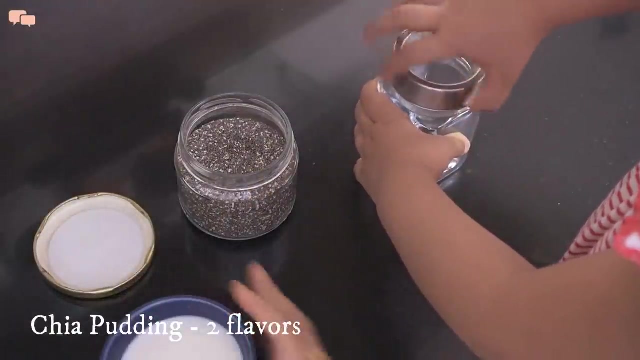 small batches, because it literally just takes 5 minutes to make a new flavour. Snacks served just in time and both father-daughter duo loved the pizza seasoning flavour. Some snacks are so underrated. Chia pudding is our favourite and always comes handy when I or Ruthvi get those hunger pangs. 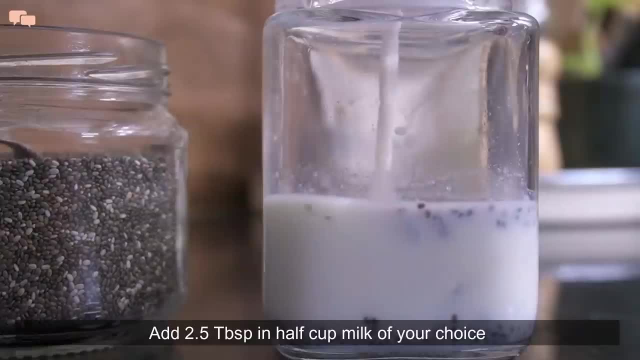 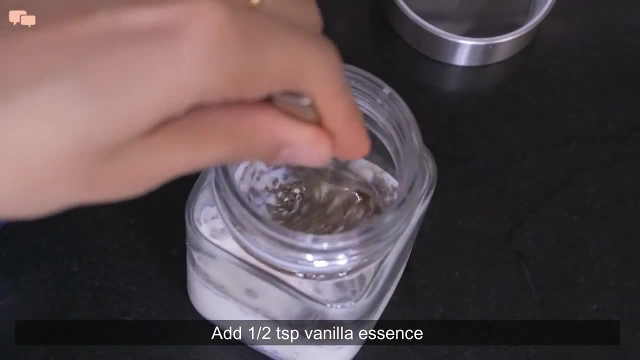 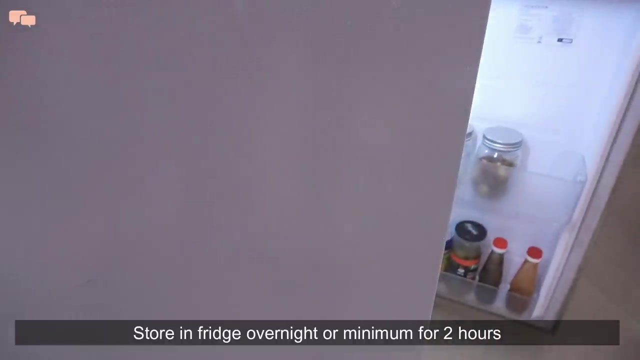 Ruthvi loves to make it and I also let her have her share of fun in creating this easy peasy snack. When kids make things by themselves, there is a low probability of them denying that dish, so it's a win-win. That's it. just mix everything together and your 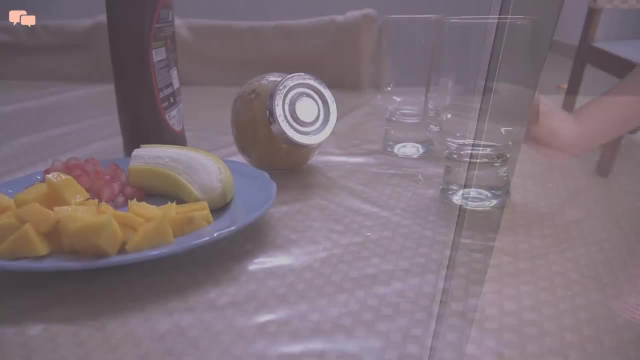 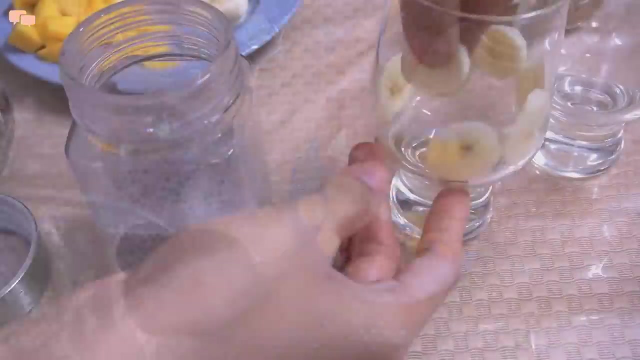 chia pudding is ready to serve. Chia pudding will be ready in a few hours. And then comes the fun part. Go crazy with the toppings, because creativity has no limit. I am making two here, but you can be as creative as you like.